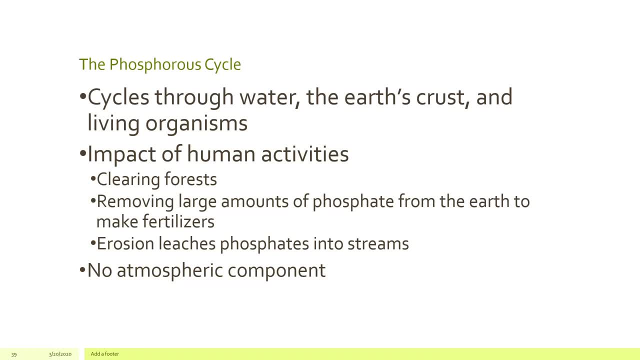 water, the Earth's crust and living organisms, And you'll notice what's the thing that it's missing. It is not part of the atmosphere. There is no atmospheric component to the phosphorus cycle. Now, human activities that are impacting the phosphorus cycle include clearing forests. 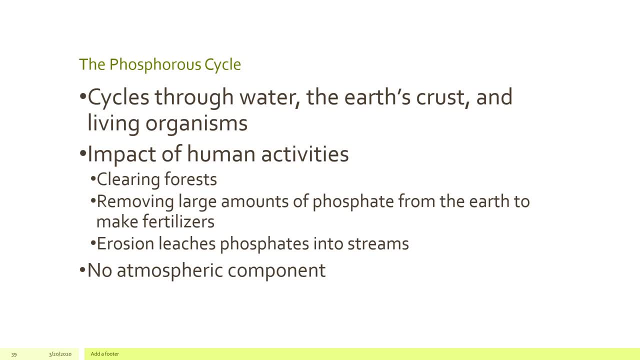 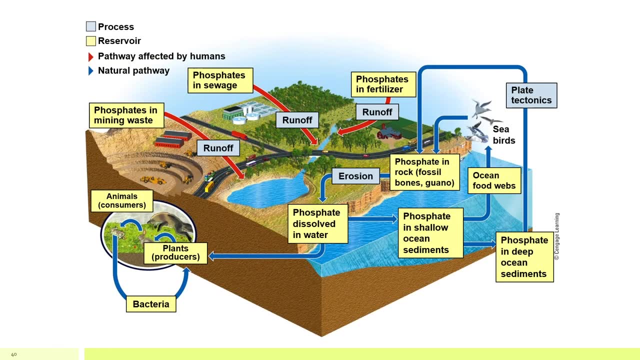 removing phosphate from the Earth to make fertilizer, and erosion which can leach the phosphates into streams. So again, no atmospheric component in the phosphorus cycle. Now, just like the last ones, we're looking at blue being natural and red being the human impact, the human cause. 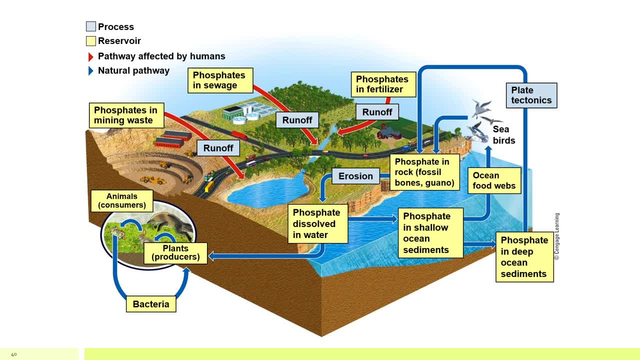 Now, for the most part, the phosphorus cycle is very, very slow. Okay, this takes a long time to get from one place to the next. Now, how are we releasing phosphorus? We're releasing it by mining waste, which comes in, runoff and then eventually gets into waterways, Sewage, lots of. 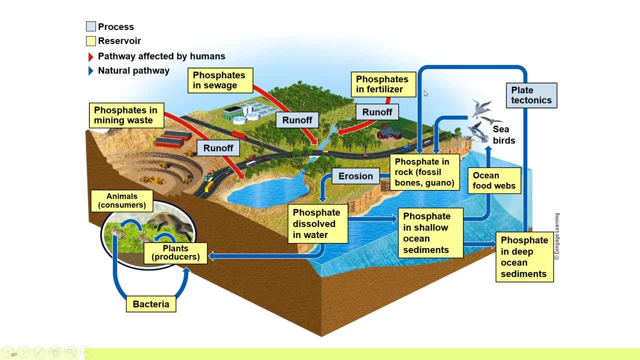 phosphorus and sewage runoff into waterways And fertilizers runoff into waterways. The natural process we will start here. we'll look at phosphate and deep ocean sediments. So way down in the ocean sediments, plate tectonics will bring that phosphorus back out and then it can be in. 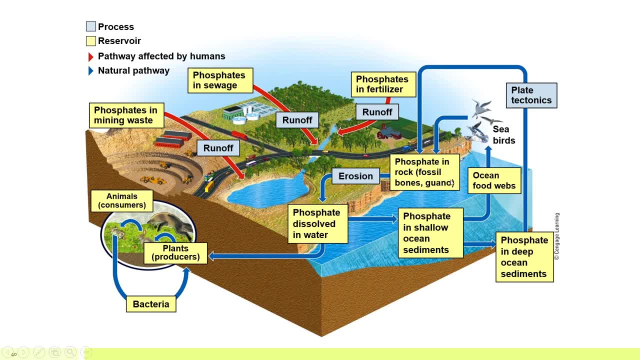 rock, So this could be fossil bones or guano. Erosion is what actually breaks that phosphate down and allows it to dissolve in the water. Now it can go from the water being dissolved in water. it can go in shallow ocean sediments eventually. 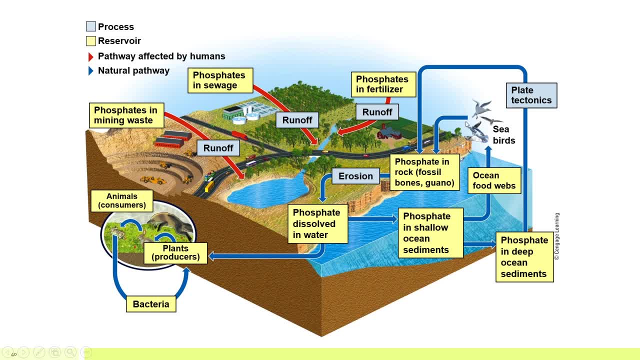 to end up in deep ocean sediments or to be used in the ocean food webs, Or it can be dissolved in water and go into terrestrial food webs where plants take it in and the animals consume it, and bacteria allows it to go from the decomposing living creatures back to the plants. So that is. 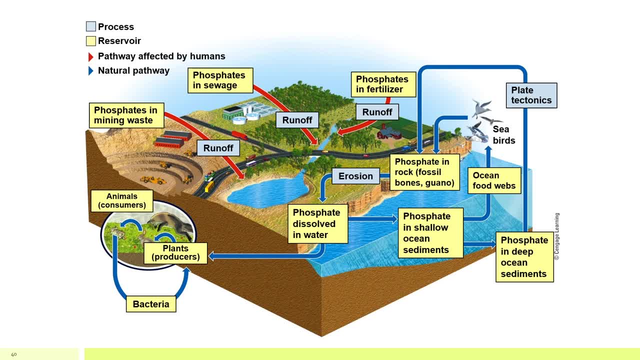 the rundown of the phosphorus cycle. Remember, very slow, no atmospheric component And, just to reminder, phosphorus is huge. when we're talking about like, why do we care about phosphorus, Why do we care about the phosphorus cycle? And it's a huge part of life, It's a nutrient For the most.